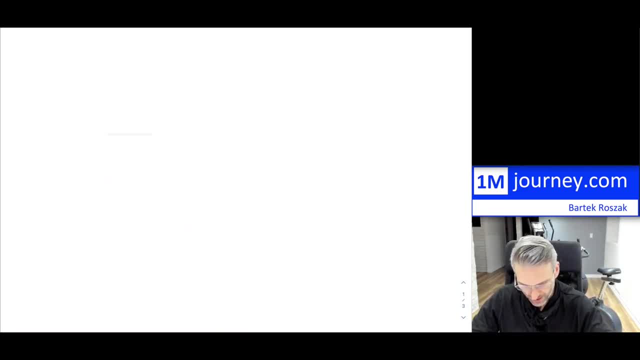 remove this for a moment so that we don't use this, because I don't want to use integration to try to convince you that it is indeed one-third. Now the convincing is going to take an assumption. the assumption is that you are familiar with the volume of a pyramid, and this just can be any pyramid with a particular 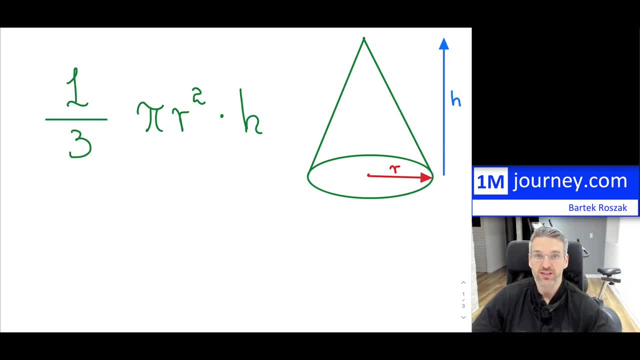 base now for our purposes. we just actually need the base to be a regular polygon, we don't need it to be anything else. now just a recall on the volume of a pyramid. so if you do take any pyramid that you have, let me just draw one quickly. 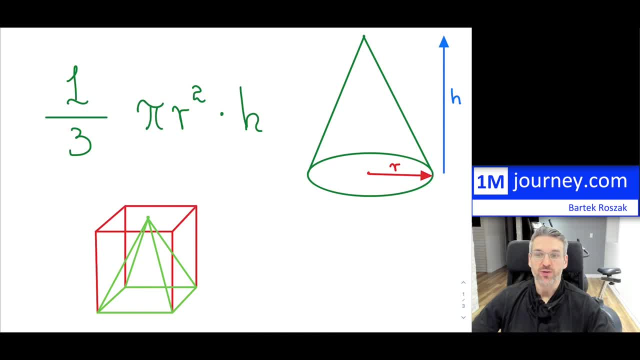 so here's our pyramid. now I've inscribed it in a prism. I can remove that prism and you can then see the pyramid. and the formula for this is indeed one-third the base, so this is the base area that we have. so let's just call this base, and 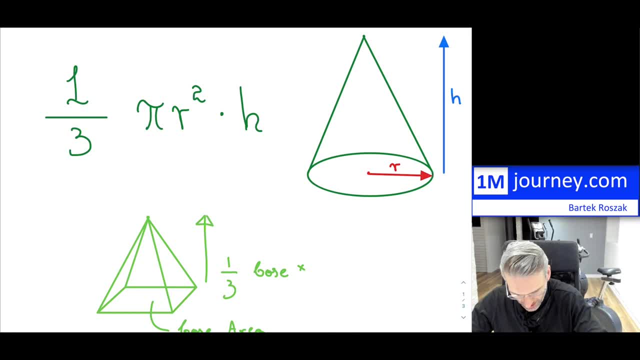 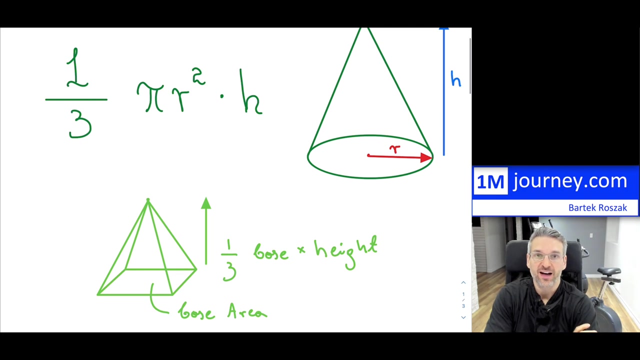 multiplied by the actual height. So this would have been the height of the pyramid. Now, if you are convinced that the pyramid has this particular volume, then you can indeed intuitively think about the cone as well. Now, if you do need convincing, I have done a very short. 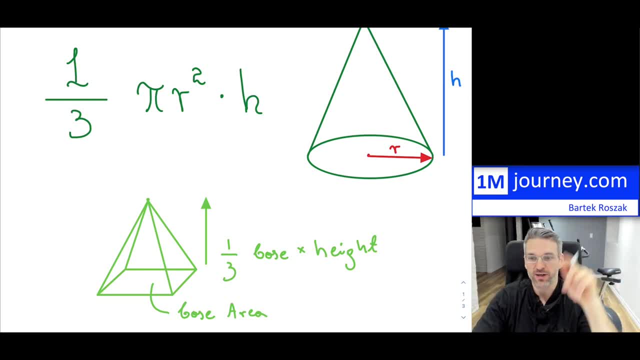 intuitive video. I can put up the link to that up above there and, for anyone who's really interested in this video, please subscribe to my channel and hit the bell icon to get notified every time I upload a new video. in trying to get the general proof, which is much longer, but I think it's. 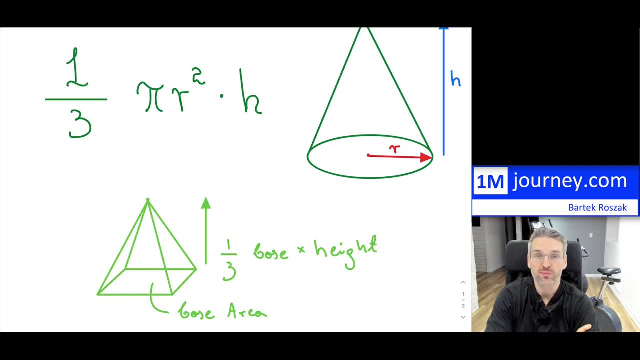 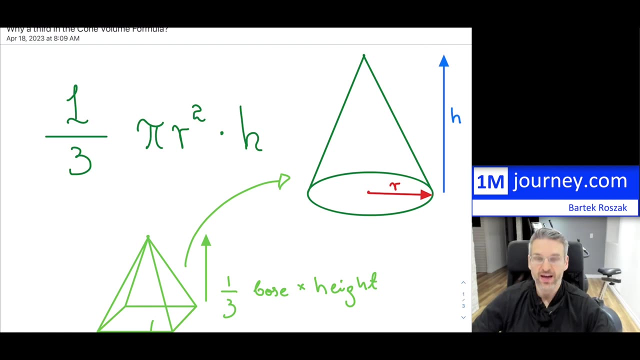 worthwhile taking a look at that for the volume of a pyramid for any base that you would like. I'll put a link to that as well. now, once we know this, then transferring from here to here is actually not that bad. now, how can you think about this without any integration? well, you can think about it. 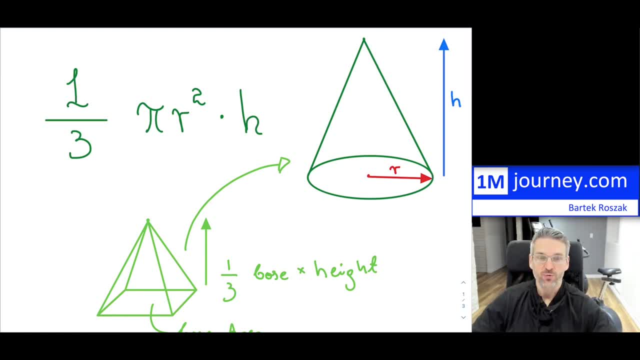 in this particular way. notice that, really, the one key item here which changes is that the cone can also be inscribed in an actual cylinder, and we know that the cylinder volume would be just the base times the height, and the cone itself is one-third. why? well, because if you take the base, which is a 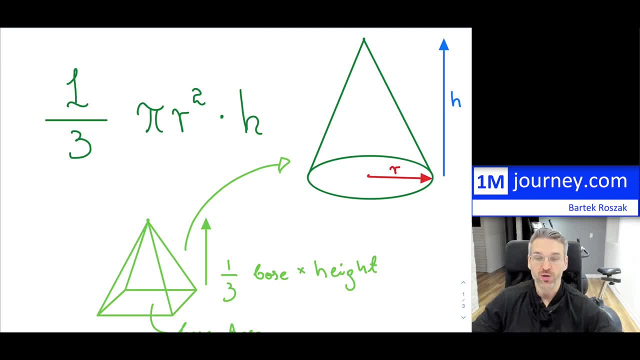 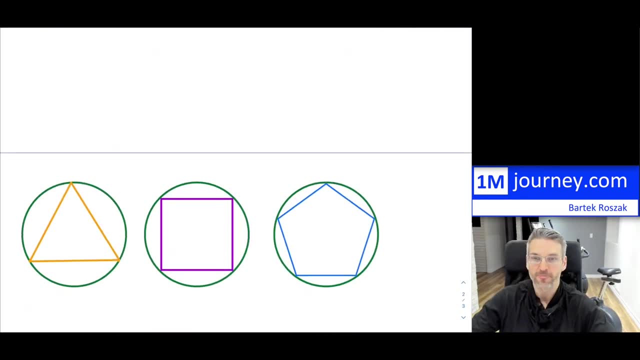 circle, and now you start taking any polygon. so notice, I'm gonna start regular polygons in here. I've kind of drew this ahead of time, you can notice, and now this is the top view, so the cone base is the circle, and then I have a polygon in here. so, for instance, I would have this: 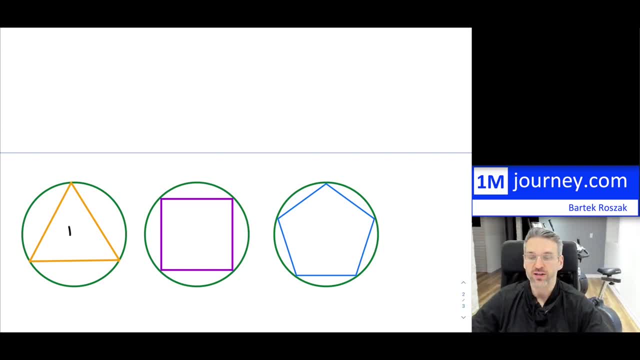 this would have been my first polygon. so it is just a base with a triangle and we know what the volume of that would be, and it's inscribed inside. now, if these are regular polygons, so the sides are all equivalent, you'll notice that now, if I extend this to a square, notice that it covers more of the circle. 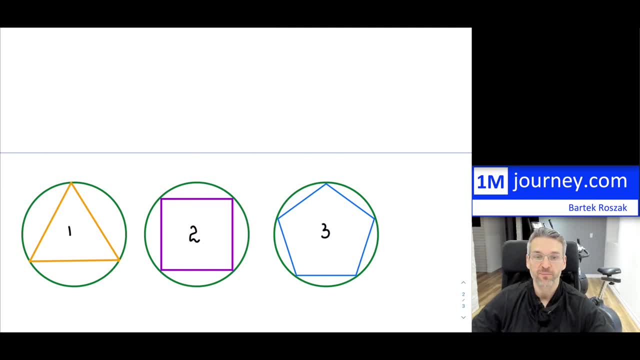 now, if I extend this to a pentagon, it's gonna be now inscribing even more, and now you can imagine this process continuing on. I could take now four sides, five sides, six sides and so on, but I'm still dealing with a polygon now. eventually, this is going to become very large. 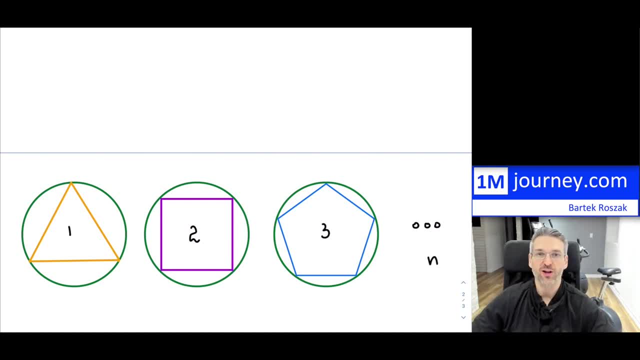 but now what happens as this becomes larger and larger and larger? well, what happens is that a polygon as n, so the number of sides, approaches infinity. as it goes to a really large number, it approximates our actual circle and if we know that, that the base can be approximated, so the actual base of a 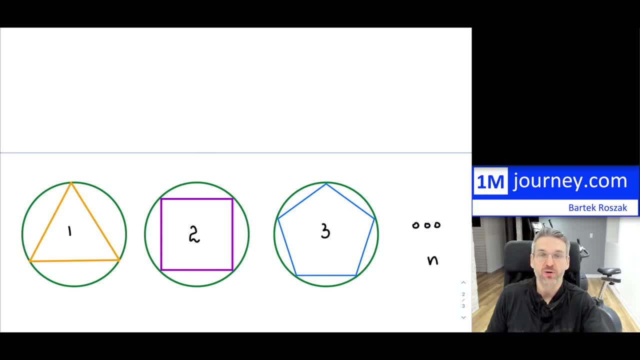 circle can be approximated by actual polygons if you take an infinite number of sides with them, and you know what the volume of a polygon is: it has a 1, 3rd times the base multiplied by its height. well then, you're done. now you're convinced. I hope that you can indeed have a cone and the 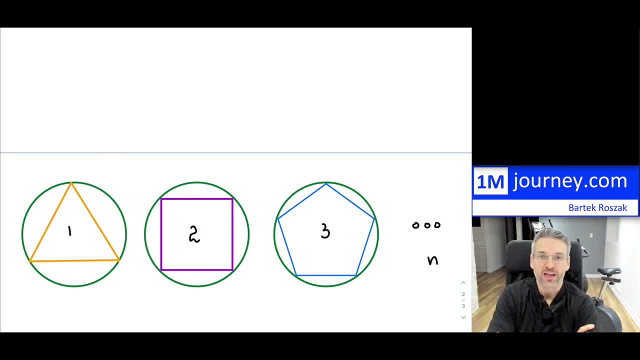 volume and that 1- 3rd makes sense because it's just an extension of the actual pyramid where the base- okay- starts to grow in the number of sides that it has. now I've actually encoded this for you and here it is. I'm using decimals to do this, but I wrote 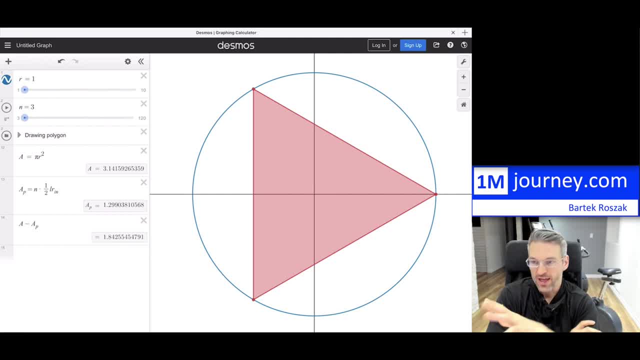 the code in on the side and you can't see all the code in here. but what I've done is I've actually inscribed a circle and then now what I'm going to do is I'm gonna hit, play on this and you're going to see, because I don't want to be. 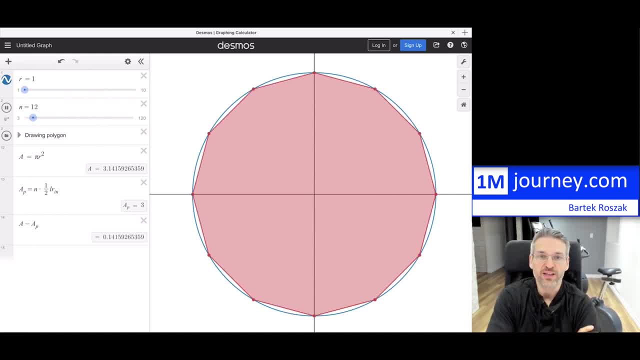 drawing all of these well, you can hopefully be convinced that as the polygon increases in the number of sides- notice here it's actually only at 22, 23, 24 and so on, so it's very little. but if you make this larger and larger and larger, so more sides- you can now clearly see, even with 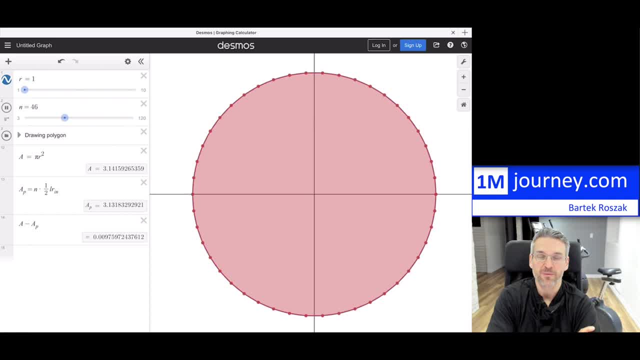 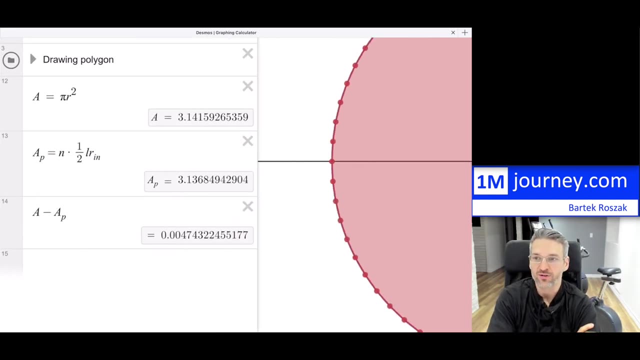 this illustration that the polygon approximates a circle. now this is from the interior and you can just keep going. now, on the left hand side of also shown you the actual areas. so notice, you have an area of your circle which is Py R squared. now I assume the R is equal to. 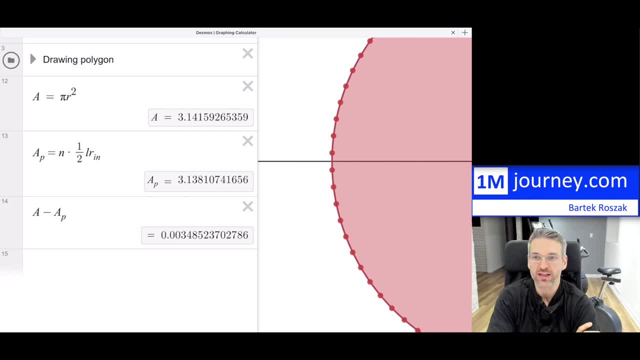 one does it matter what it would be, but one is convenient, but it again, it is irrelevant. and notice that just below it there is the area of the polygon as it's increasing. now notice what it's tending to and at the bottom, which is the area. 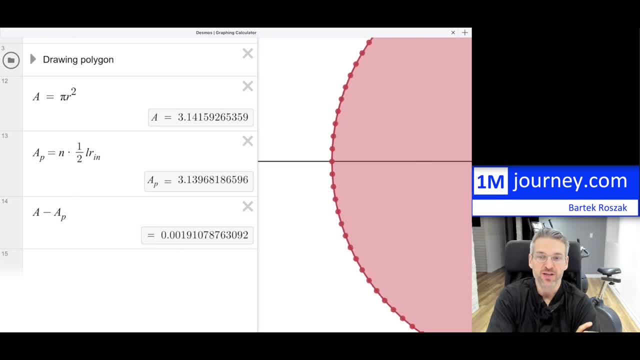 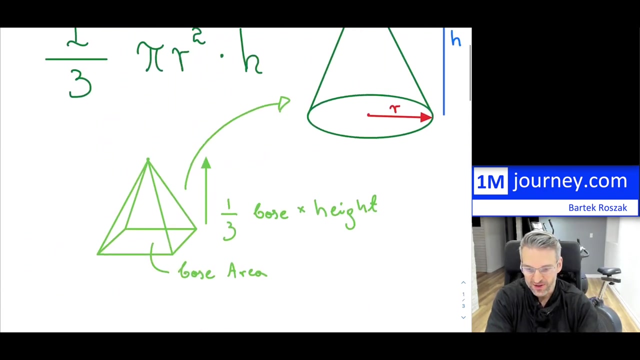 of the circle, the area of the polygon, notice that the difference between them just gets smaller and smaller and smaller. why? because the polygons- okay, as n tends to infinity- basically create a circle for us, and so from that we can actually conclude that, indeed, intuitively, this one third. 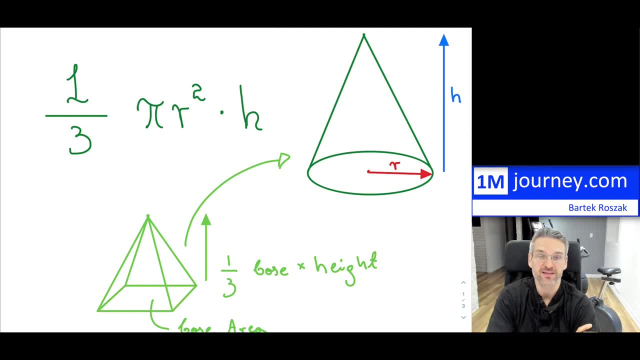 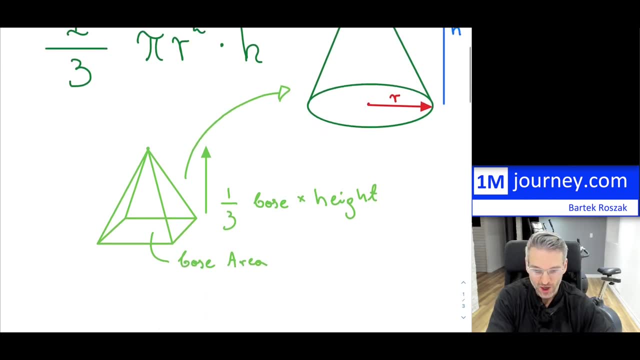 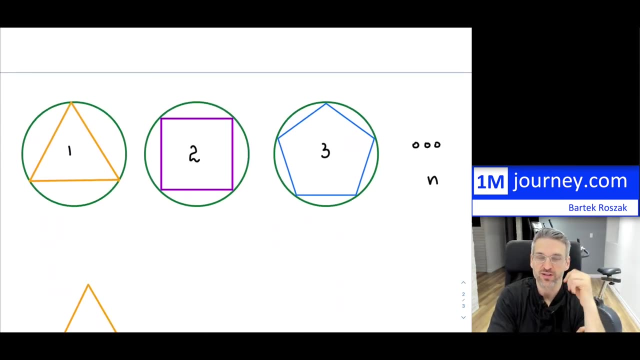 for the cone completely makes sense. it's just an extension of pyramids. that's all that it is. now, to be completely honest with you, this still uses some part of calculus because it uses limits, as n tends towards infinity is basically a limit, and if you really wanted to show this, you can't. 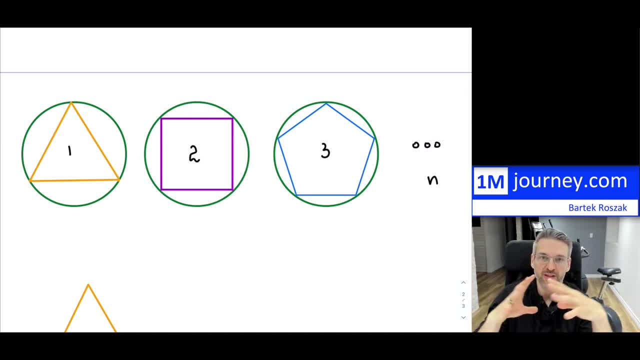 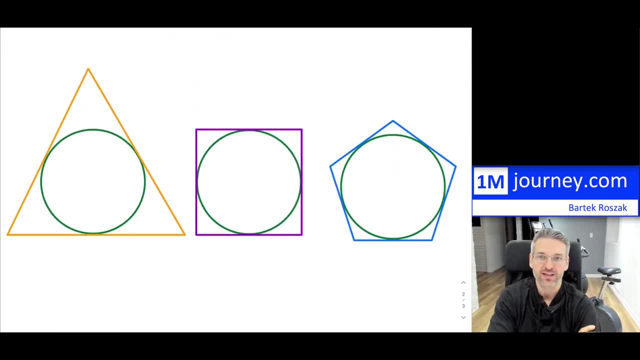 just show interior that it encapsulates and basically approximates a circle. you can't just show interior that it encapsulates and basically approximates a circle, that it encapsulates and basically approximates a circle. You also would have to do the same thing from the exterior. 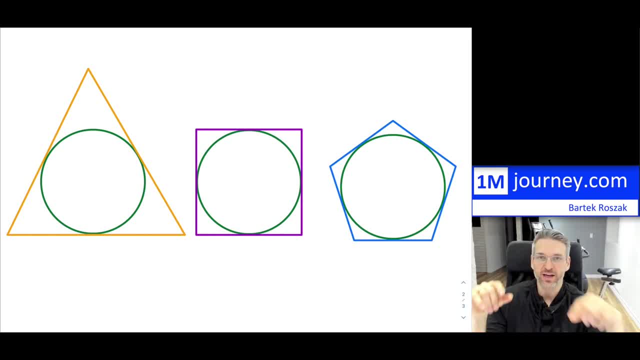 So meaning, as you can see here, you can now create a bigger triangle And that triangle encapsulates the circle inside. Then it goes into a- well, a square. That square encapsulates the circle, But look what happens. then it gets into a pentagon. 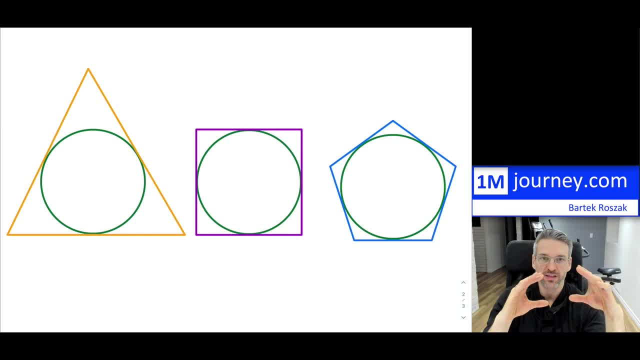 And notice that our polygon just gets smaller and smaller and it gets closer and closer to the circle. And in the illustration that I did in the simulation, I didn't do both of them, but I did the one on the interior where it approximates it from the inside. 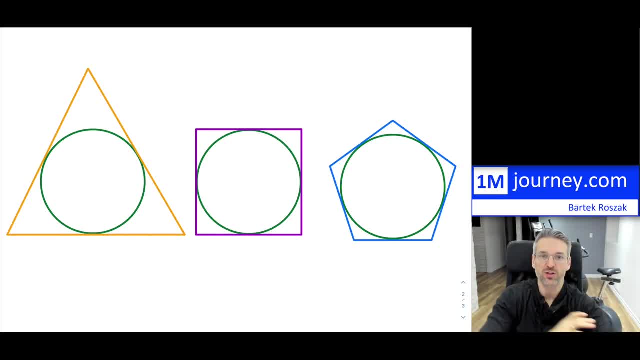 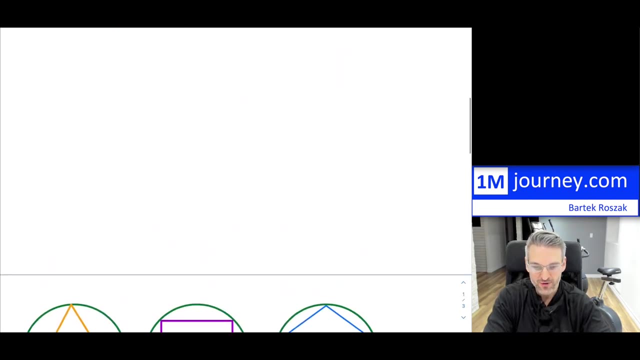 and it also will approximate it from the outside, which is going to engulf and basically have a circle. Now, this is a particular theorem actually used from limits, but you don't need to know it. Hopefully this convinces you that, indeed, the area that we have, or the base itself, 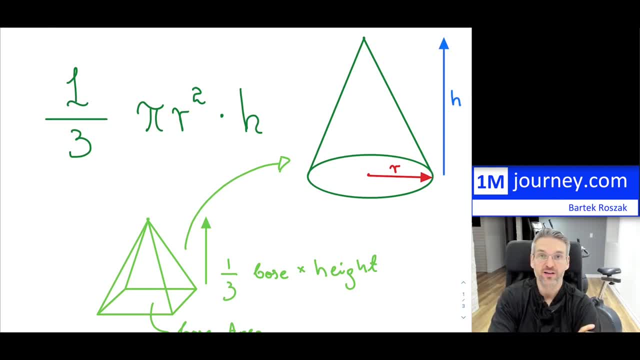 can be approximated by polygons And we know what the volume of a pyramid is with a base of a polygon. And there you have it. That's why we have one third of the actual cylinder existing in our formula, intuitively, without any integration. 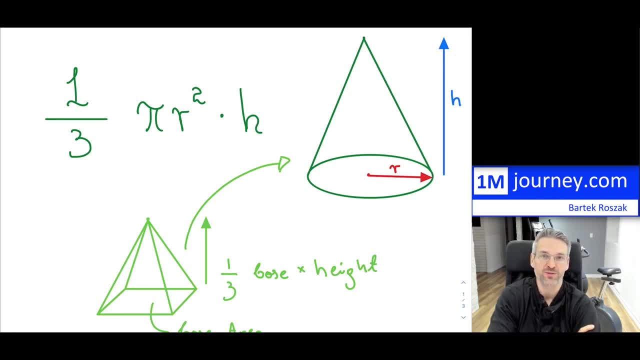 but hopefully a convincing visual representation for you. Thanks for watching. okay, Give it a thumbs up if you liked it. We'll see you in future videos. Bye, welcome to onemillionjourneycom, cheers.